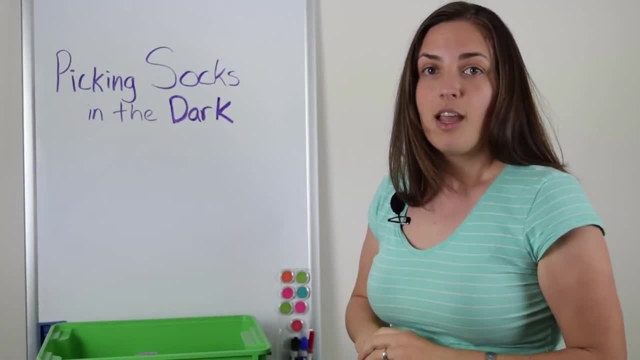 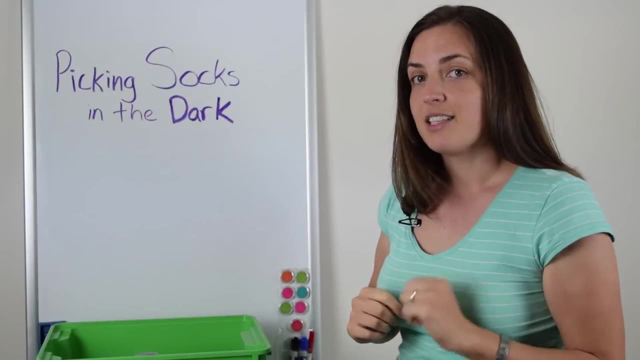 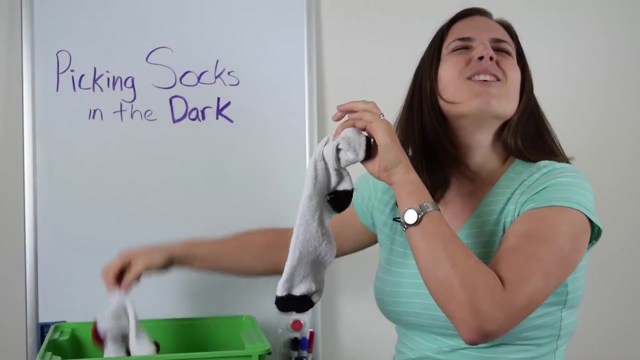 socks and be guaranteed to get a matching pair. So I'm going to do this with my eyes closed, so you know I'm not looking into the box and I want to know how many do you think I need to pick? So let me start Close my eyes. I don't know what this is and I don't know what this is. 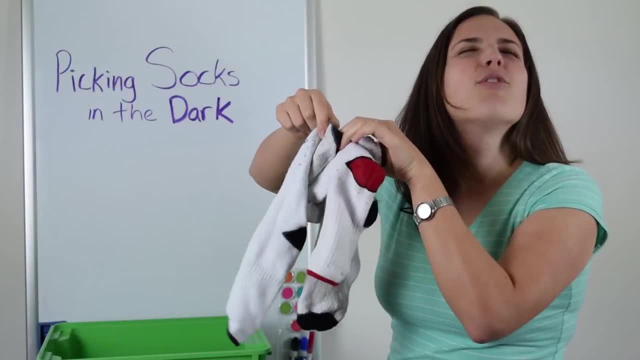 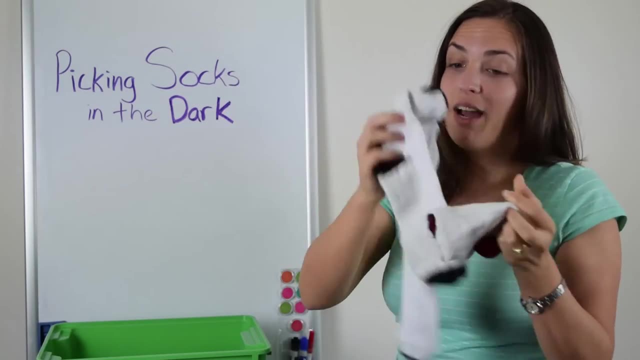 and I don't know what this is, but I've only done three picks And I'm going to stop. Well, I happen to pick all three white in this case. So I do have a matching pair and in this case I can even call this a matching pair because, remember, I'm ignoring the 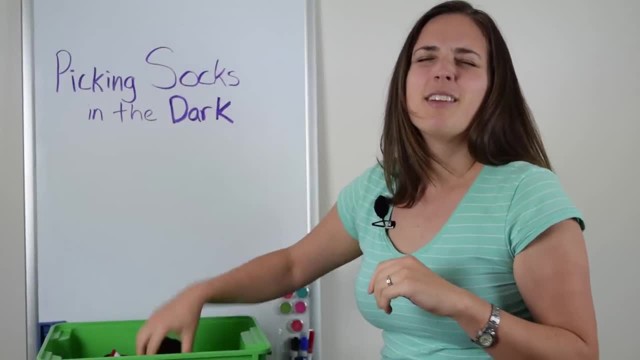 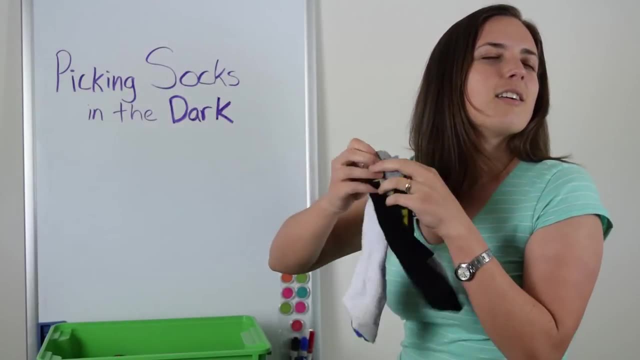 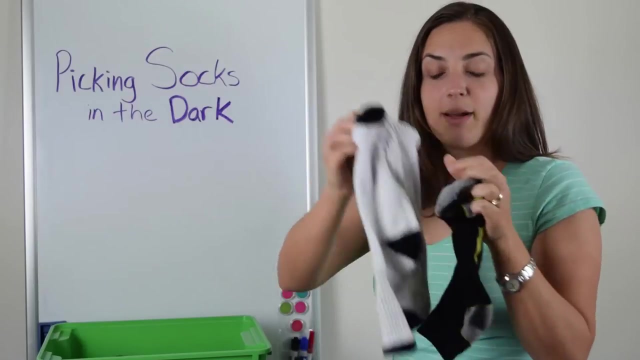 colors. Let me do this again. I'll mix them up again and I'm closing my eyes and I'm looking away and I'll pick a sock, and I'll pick another sock, and I'll pick another sock, and I look and I got a black and two whites, but again I have a pair. 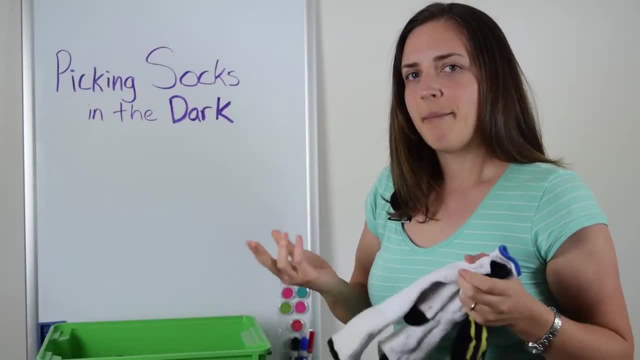 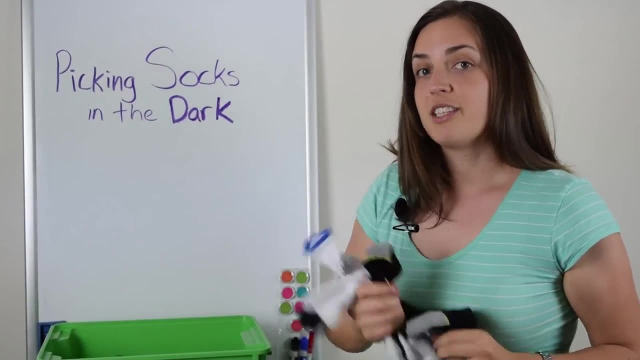 Now notice that I always stopped when I only picked three socks. Why am I doing that? It turns out you are always guaranteed to get a matching pair. if you have two colors, You only need to pick three socks. Why does this work? Well, it's because of the pigeonhole principle, So let's write that down. 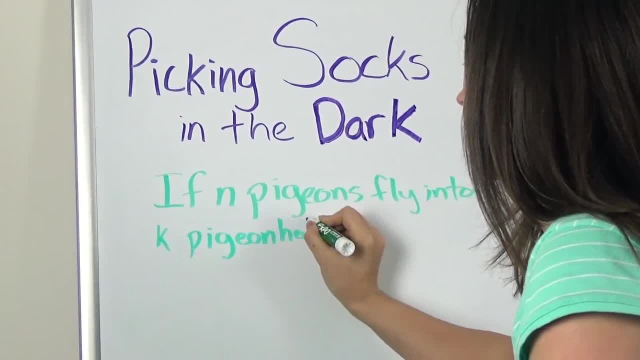 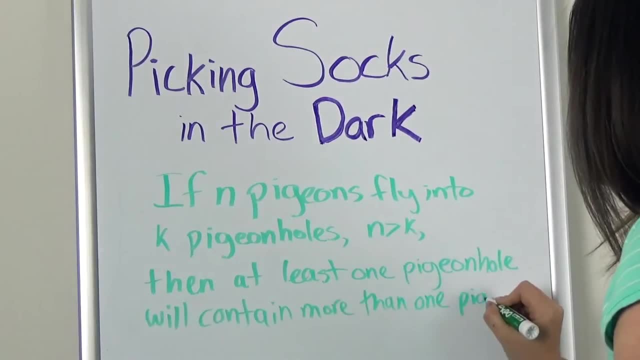 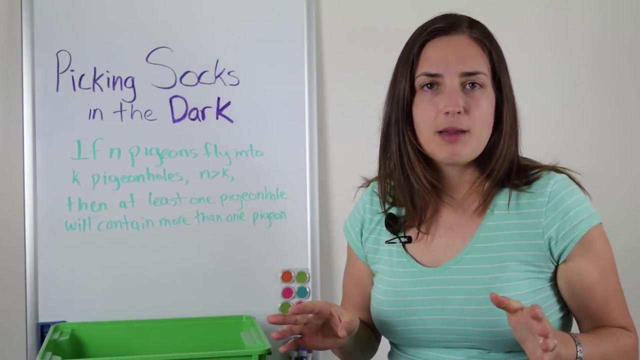 If n pigeons fly into k pigeonholes where n is bigger than k, then at least one pigeonhole will contain more than one pigeon. Let's think about why that is true. So let's say you have three pigeons and they need to fly. 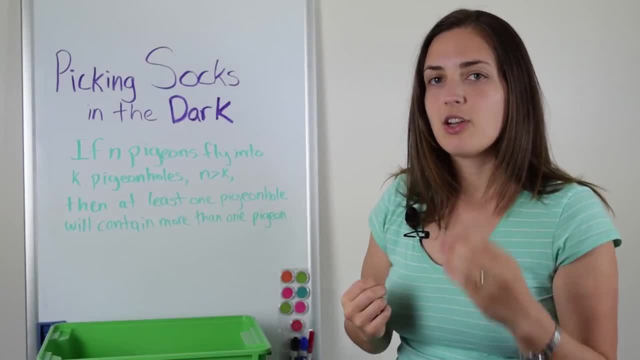 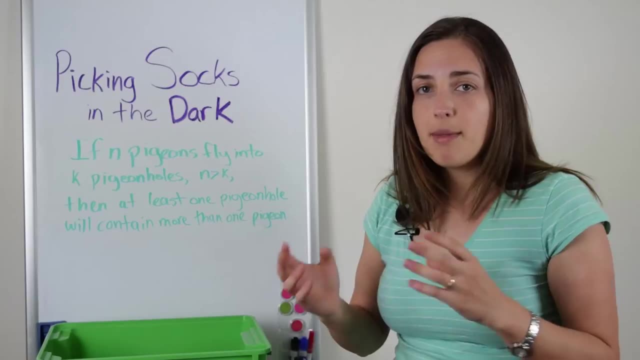 into two pigeonholes. So in this case n is 3 and the number of pigeonholes k is 2.. So we know that 3 is bigger than 2.. If they're trying to fit into two pigeonholes, maybe all three of them go into one hole and none into the other, or 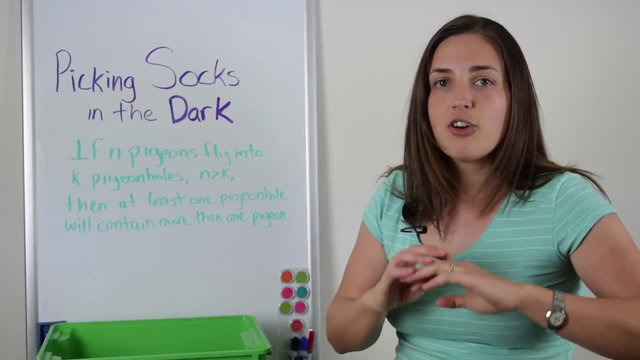 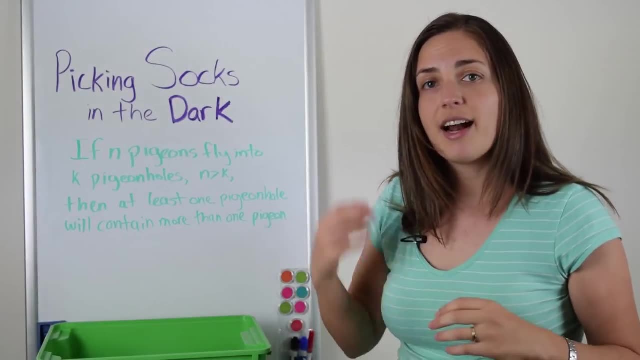 two and one and one and the other, but you're guaranteed that you're not going to have every pigeon individually by itself, because there's just not enough pigeonholes, So you will have at least one pigeonhole that has more than one pigeon. Let's imagine this with ten pigeons. Let's say we have ten pigeons. 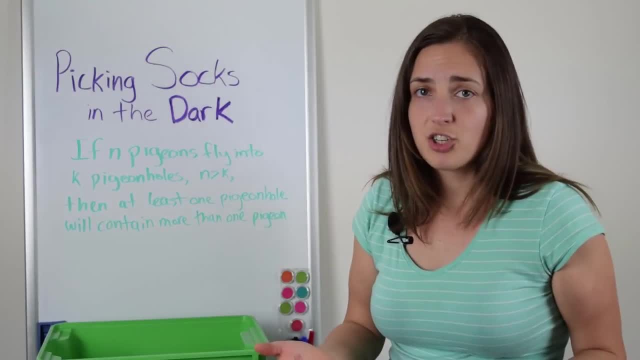 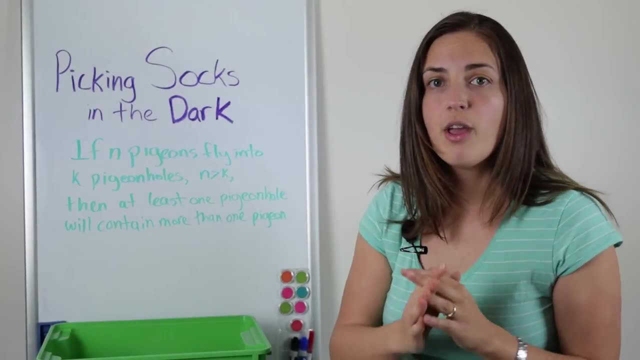 and nine pigeonholes. You try to put all those pigeons into the pigeonholes and there will have to be at least one hole that contains two pigeons. Now there might be a hole that contains five pigeons, we don't know, but there is.